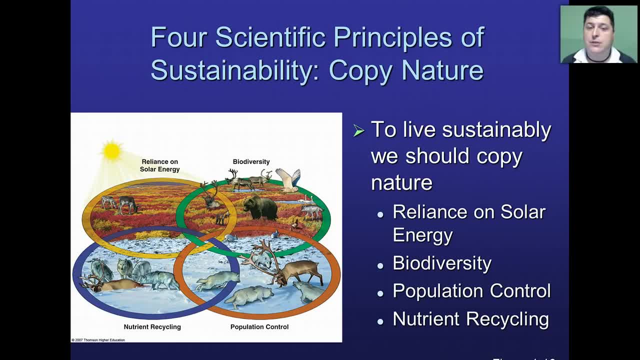 And so perhaps, if we mimic nature's ability to be sustainable, we also can be more sustainable. So there's four basic principles from nature that we might be able to borrow in order to live more sustainably. The first one is reliance on solar energy. 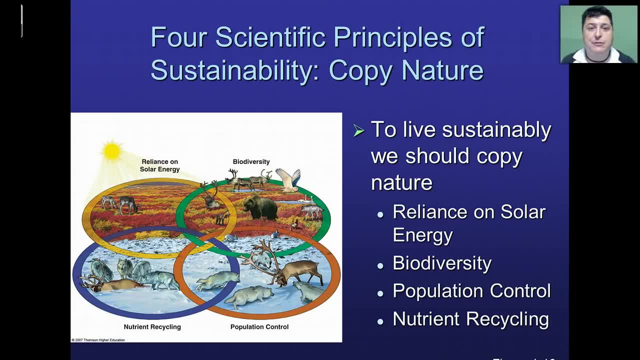 Nature uses the abundant perpetual energy source of the sun. The sun produces no residual pollution and it's an endless source of energy. So if we can find more ways to use solar energy, both actively in the production of electricity or hydrogen, or passively for the heating and cooling of our homes, we could live more sustainably. 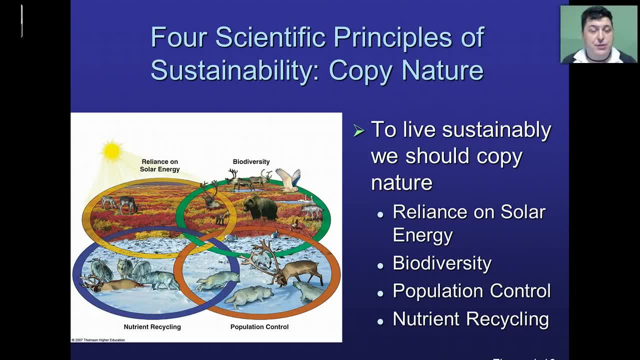 Another one is: nature relies on biodiversity. There are organisms that provide services and produce things in the environment. Each organism has a role And there's lots of organisms. There's a diversity of living things, So if one happens to naturally go extinct, there's hopefully somebody else there to do its job. 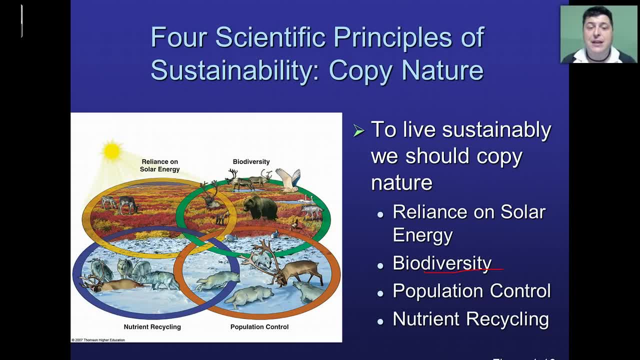 So we need to maintain that biodiversity to make sure that there's plenty of living things that are providing those natural resources for us to be able to survive and maintain our economies. Another thing is population control. In nature, living things rarely exceed their maximum amount of organisms that can be sustained in a given area. 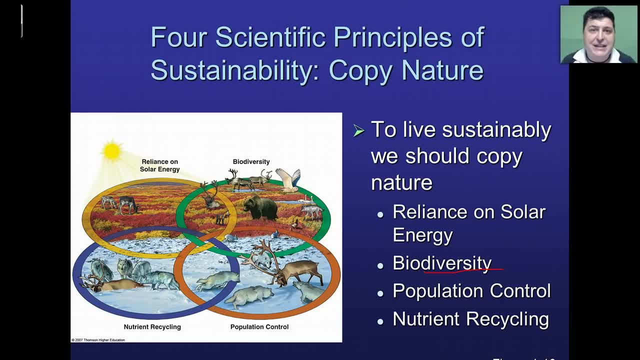 And even if they do go over that bump, they're always brought back down to an appropriate level. Humans, because of medicine and our knowledge of technology, we've been able to really grow as a population exponentially to over 7 billion people. Is that too many? 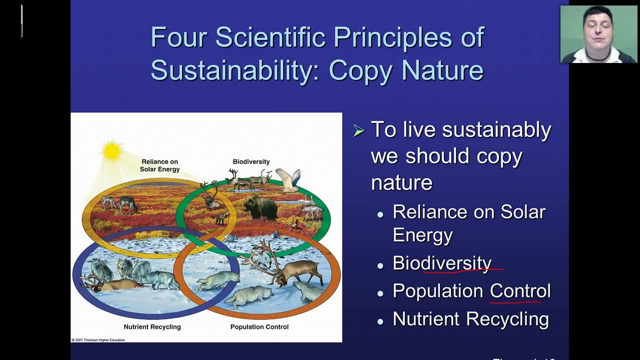 Should we Think about some ways that maybe we can try to manage our population so that we're not taking too many resources? And lastly, nutrient recycling In nature. nothing is wasted. Everything goes back to nature. The first law, or the law of conservation of matter, says that matter can't be created or destroyed. 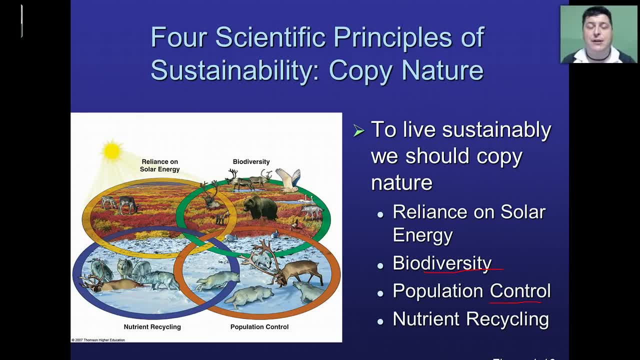 So nature is going to rely on that so that each piece of matter can be recycled. If you've had physics, you might recall that talking about all of the matter that is present on planet Earth was here at the formation of our planet, And so the atoms that make up our bodies have been recycled for thousands and thousands of years. 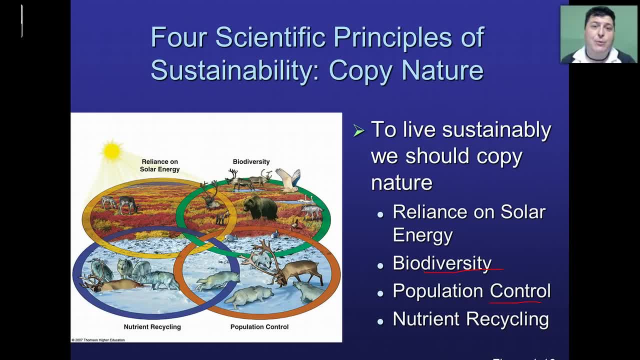 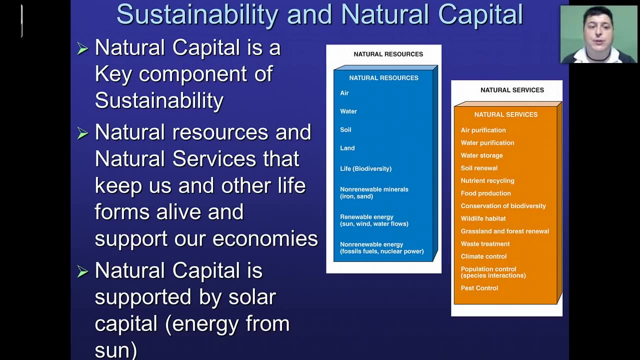 Our matter has been recycled, And so when we're producing goods and making waste, we need to consider how we can recycle that and make sure that we're mimicking nature. Now, the key to sustainability is understanding the resources, the resources that we're using, and that those resources are what we call natural capital. 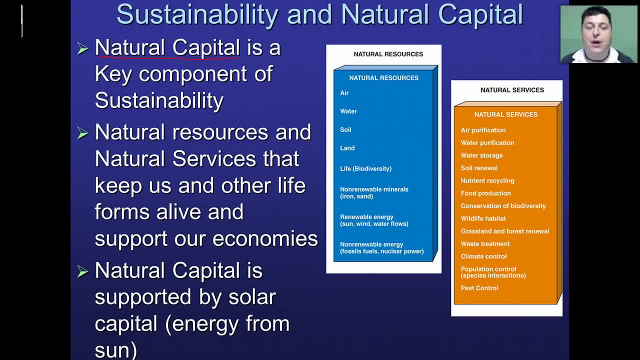 And when we think of capital, oftentimes we think of, you know, Capital One, commercials and capital in terms of money, money that we spend. Well, natural capital are those things that we're going to use, we're going to spend in order to maintain our livelihood and our economies. 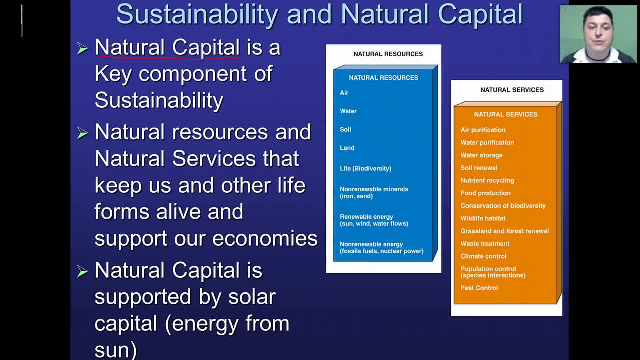 The two big pieces of natural capital are natural resources and natural services. Natural resources are the things that are present in nature or that are produced in nature that we're going to use. Okay, things like air, water, soil, land, the living organisms, minerals and energy sources. 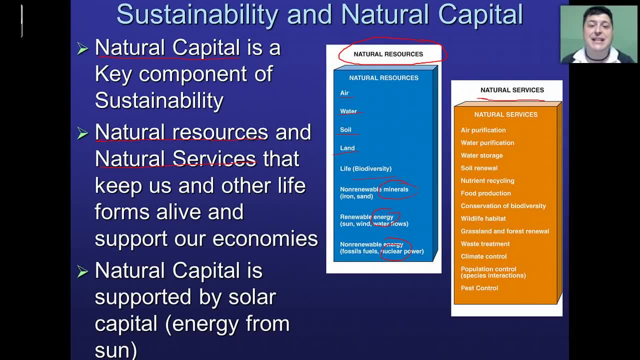 While natural services are the processes, the things that nature does. that also is going to produce something for us, like cleaning our air or making some food or breaking down waste and recycling that matter. Now, what keeps natural resources forming and natural services do it being produced is going to be the sun. 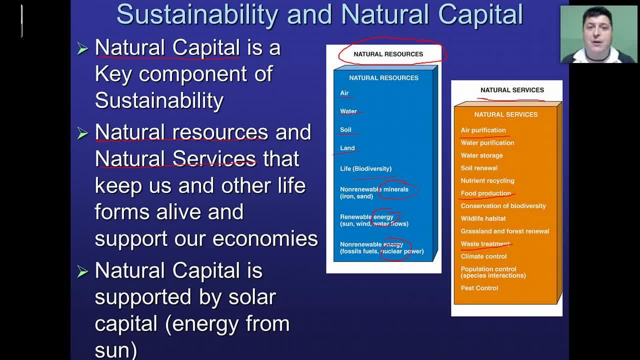 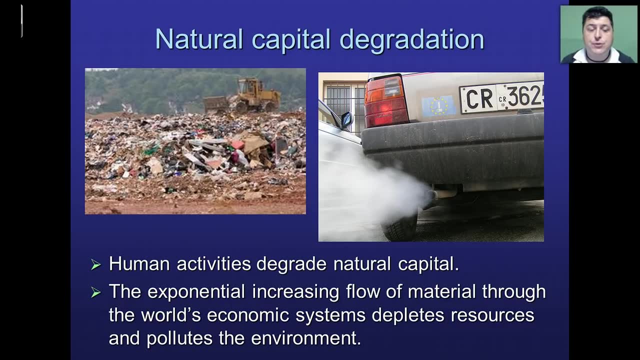 The sun is one of the major driving forces to a lot of natural processes, And so we say that natural capital is supported by solar capital, solar energy. Now, as we consume natural capital, as we produce, we consume natural resources, As we produce items and make waste, we say that the capital is being degraded. 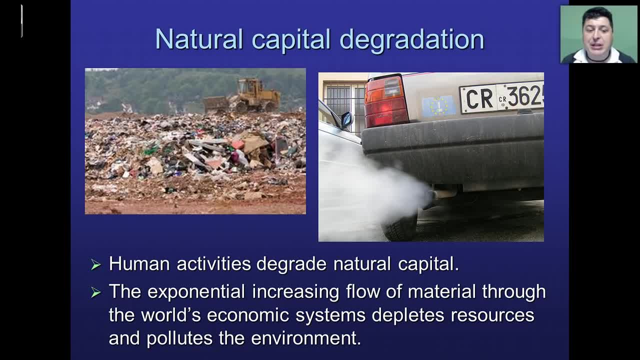 We're spending those resources, So we're depleting resources and polluting the environment, And if we're going to be sustainable, we need to find a way, find that balance, so that we degrade less of that natural capital and use it more efficiently. 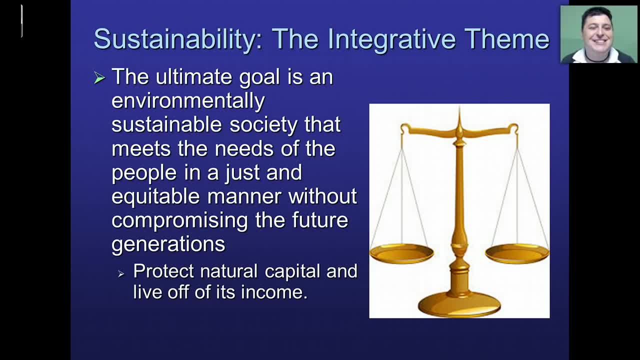 So that our ultimate goal, then, is to create an environmentally sustainable society, one which is able to meet the needs of all people. So that our ultimate goal, then, is to create an environmentally sustainable society, one which is able to meet the needs of all people. So that our ultimate goal, then, is to create an environmentally sustainable society, one which is able to meet the needs of all people, And do it in a very just and equitable manner, without compromising our future. And do it in a very just and equitable manner without compromising our future. 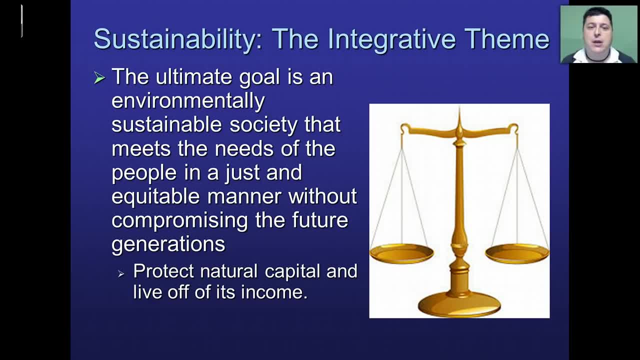 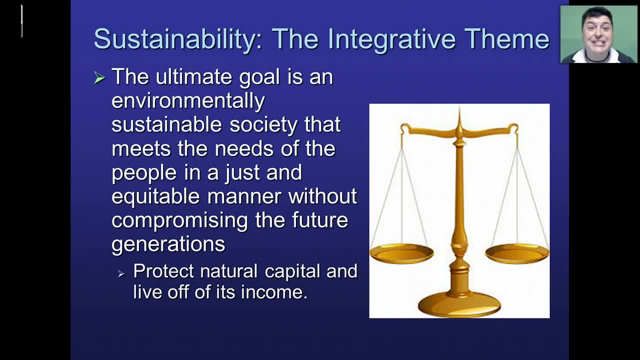 So we want to make sure that we're protecting our natural capital. So we want to make sure that we're protecting our natural capital. So we want to make sure that we're protecting our natural capital. We're saving some of that capital and living off of its income. 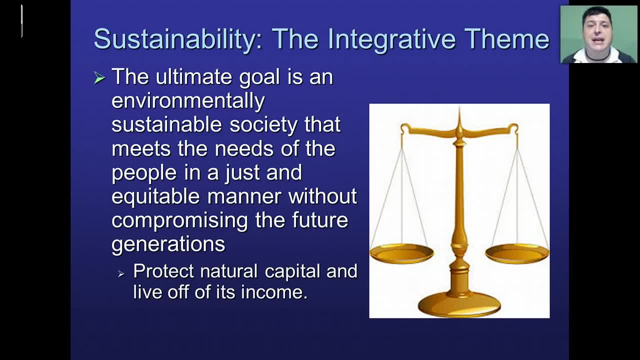 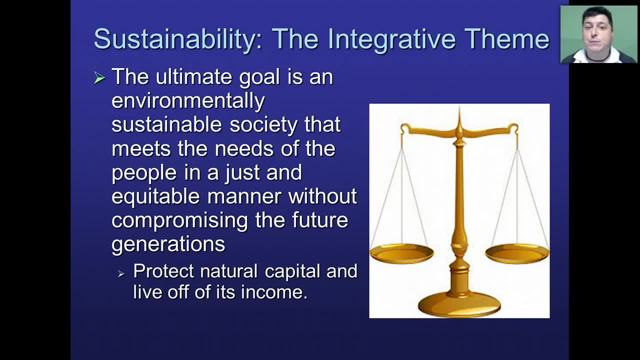 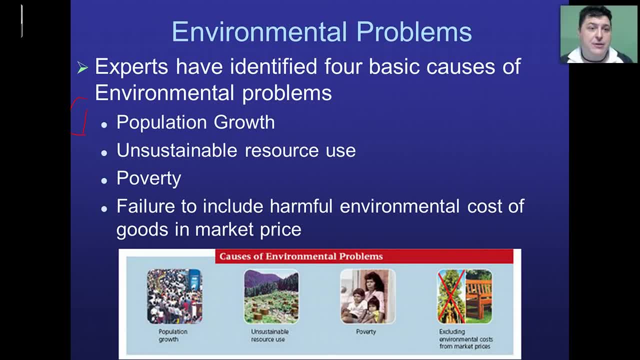 earth and more coming every day, more than are dying. we have lots of people, and each one of those people require resources and they're going to impact the environment, and so we have to think about how we can manage our population. we use our resources very much, unsustainably. we've become especially in 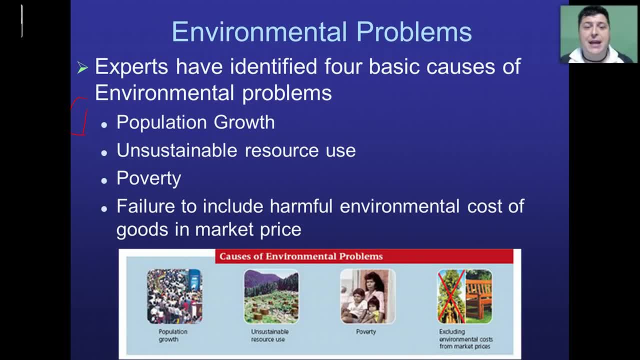 the United States, a disposable society. we throw so much away that perhaps can be reused or recycled and we can use our resources much more efficiently. number three is poverty, something that we have to work on. when you have nations which have a low gross national product and the individuals don't have a lot of 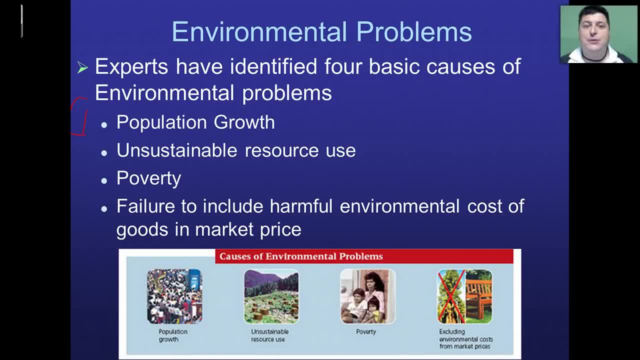 money to spend. it's hard for a person to consider using resources efficient, efficiently and paying for good disposal of waste when they have a hard time putting food on their table. and, lastly but not leastly, we have our failure to include harmful environmental cost of goods in a market price. in other words, when a product goes to market, the 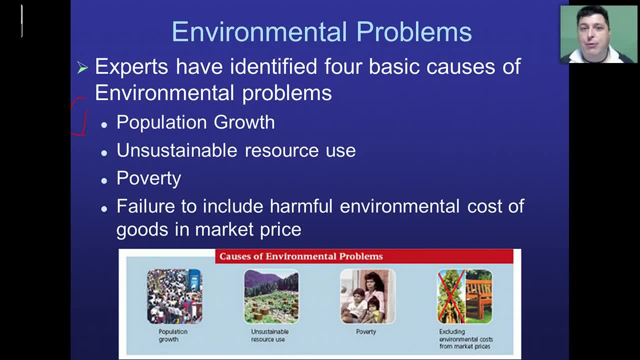 impact that it had on the environment is not included in the price. for example, if we have a piece of furniture that was produced from wood from a rainforest versus a piece of furniture that was produced from a sustainable forest in the Midwest, both pieces of furniture may be identical in their form. 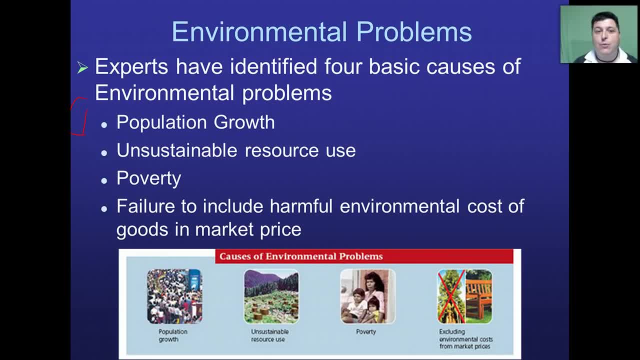 and they will have an identical price, even though wood from the rainforest damaged the environment much worse, because it was not harvested in a sustainable manner, whereas the midwestern forest has a sustainable harvest, that's associated with it. If the rain forest piece of furniture cost more, 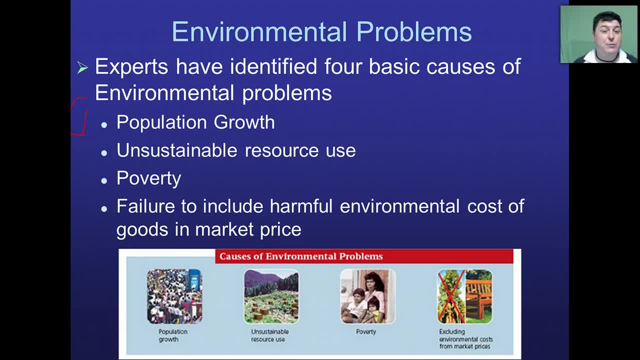 than the one produced sustainably. a person will be less likely to buy that, and that would discourage unsustainable forestry practices, perhaps. So if we had to pay for our impact on the environment, it might change how we consume goods. Now there are a lot of different solutions. 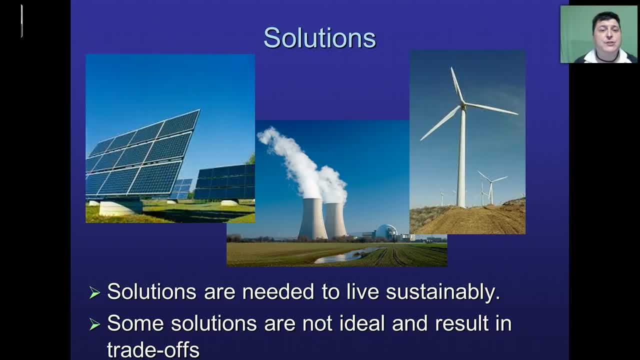 to environmental problems. Unfortunately, there is no panacea. There are some solutions. in fact, all solutions are going to have some sort of trade-off. Solar energy is great because the Sun is a perpetual energy source. It's clean, virtually non-polluting. The problem is: 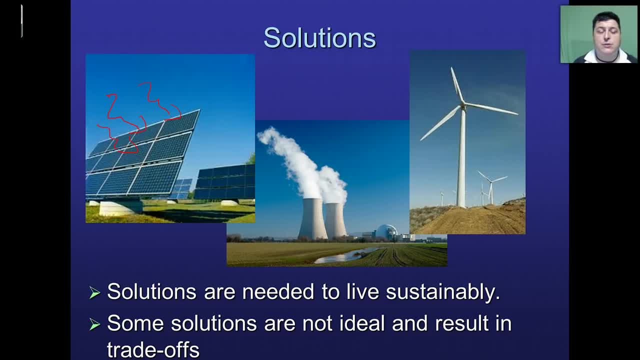 there are only certain areas which are really optimal for solar energy and in some cases, when you're placing that solar panel, you might be disrupting a habitat for an organism. Nuclear energy is very low in its carbon emissions, but we have this leftover, nuclear waste. How do we deal with that? Wind is a good solution. It's. 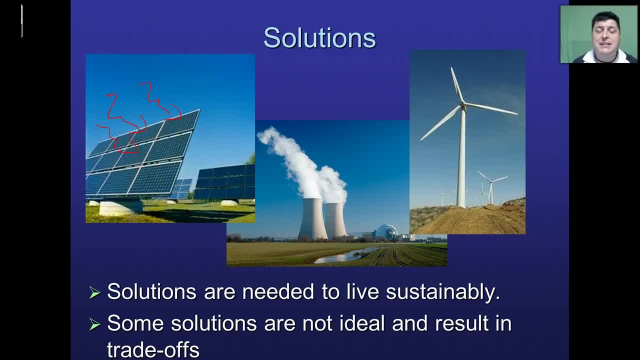 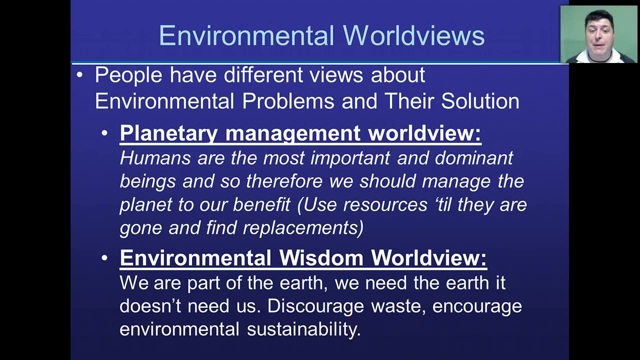 also virtually non-polluting, but it does sometimes emit noises which can be annoying to people. It can disrupt flight patterns for birds, So it's not a perfect solution. People have different views about the environmental problems and their potential solutions. They range from the planetary management worldview, which says that humans are the 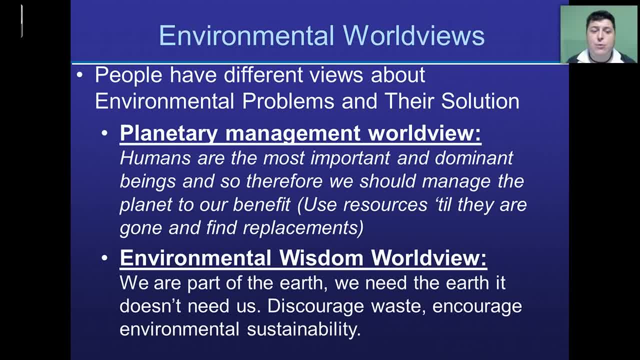 most important and dominant species on the planet. so we should manage the planet for our benefit, Use those resources until they're gone and then find a replacement. Let science solve the problems. The other end of the spectrum is what we call the environmental wisdom worldview, which says that we're part of. 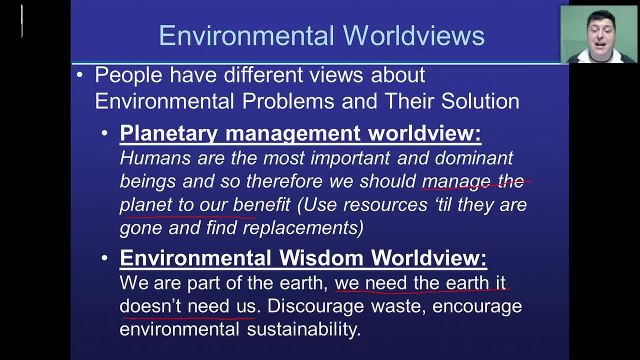 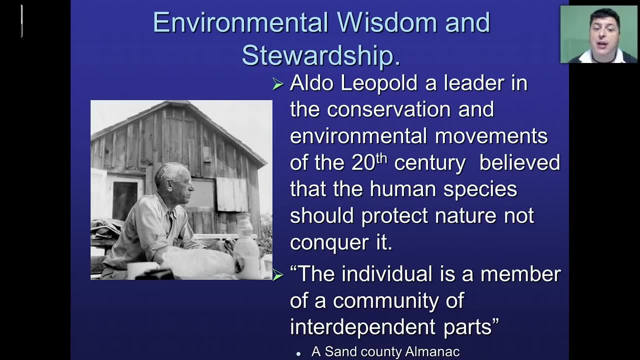 the earth. We need the earth. It doesn't need us. So we should manage it appropriately, discouraging waste, encouraging environmental sustainability. A champion of the environmental wisdom worldview was Aldo Leopold, who was a leader in the conservation environmental movements of 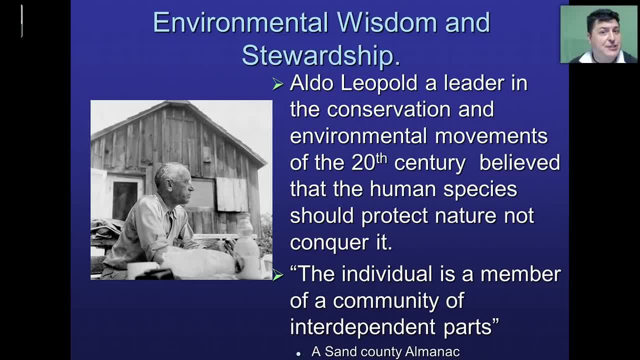 the 20th century and he believed that human species should protect nature and not conquer it. He purchased 80 acres in central Wisconsin and put principal tools of sustainability into practice. He took a tract of land that was over forested and over harvested and restored it. His efforts were, he recorded. 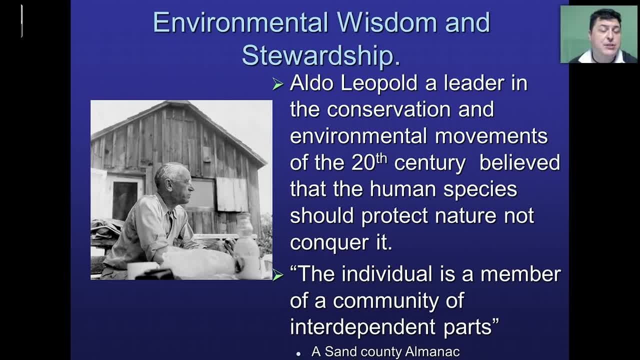 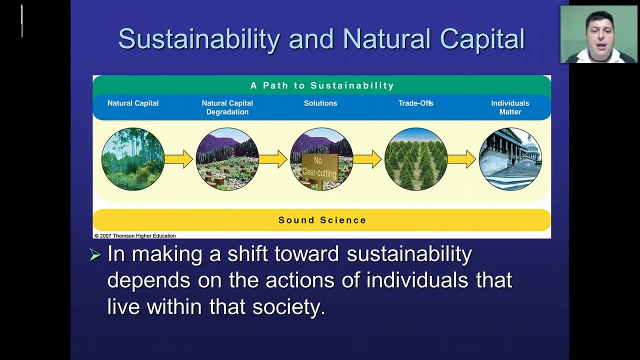 in his book called A Sand County Almanac, which was published shortly after his death. In it he stated: and the individual is a member of a community of interdependent parts. We're all connected with the earth and so we need to take care of it.